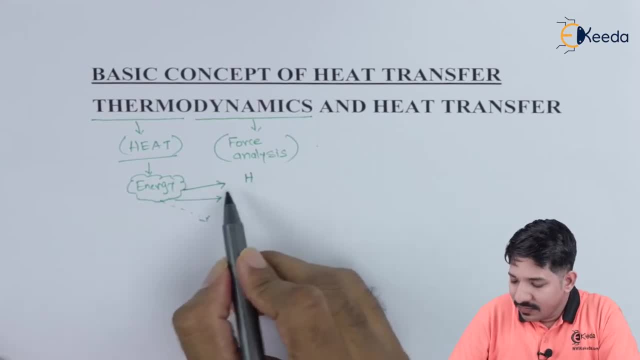 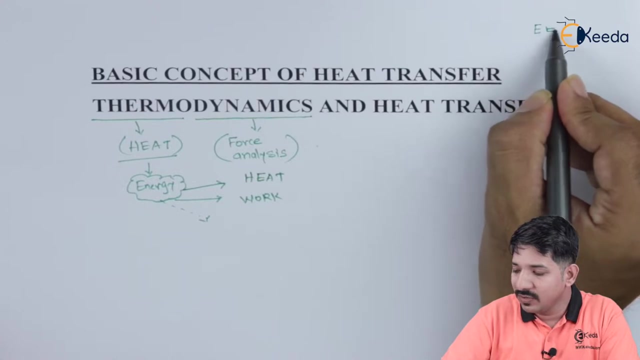 are going to do the force analysis In thermodynamics, the energy. we had three forms of energy. First one is heat work and then the last one is something that is very new that we have learned thanks to the great Einstein. Because of him, we got to know E is equal. 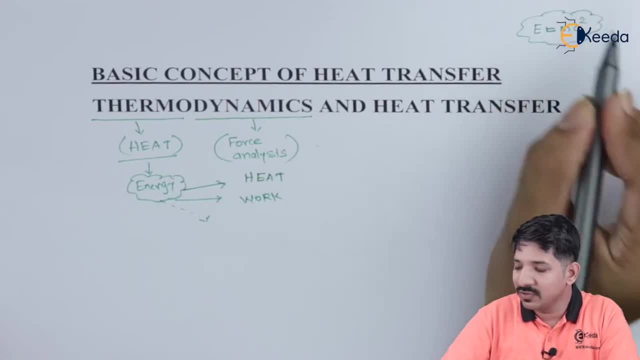 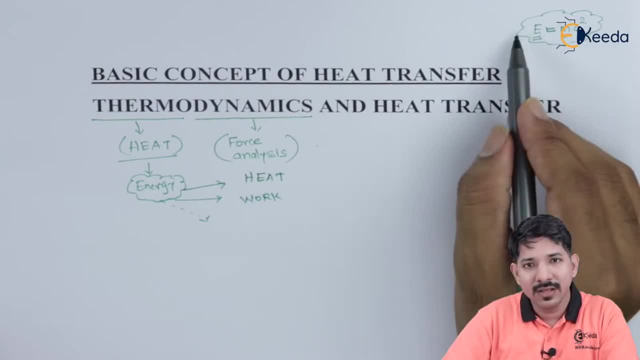 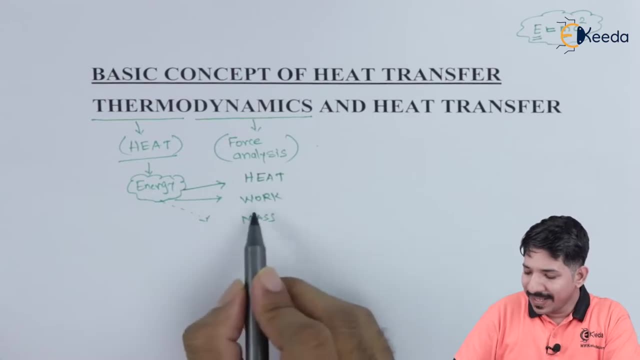 So we are going to do the force analysis. So now lets see. So we are going to do the first part, That is, the energy and mass itself can be inter connotable. That is why what we can say is: mass itself is a form of energy. But anyway, 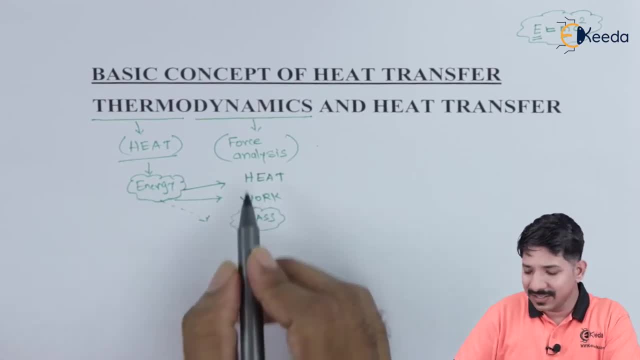 we are not going to consider mass as a form of energy in the thermodynamics syllabus. We only consider the heat and work. So we tried to understand that there is something called heat and then there is something called work. This we try to understand from the concept. 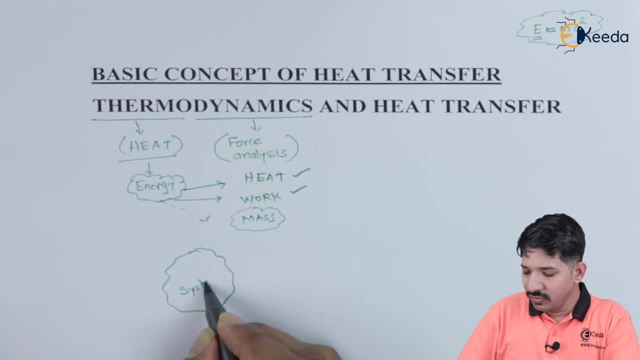 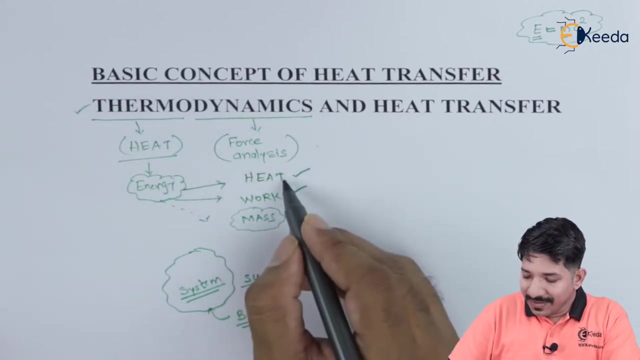 of system and surrounding. So we used to focus on some space in a given region. now that space we call as system, and something that separate the system and surrounding is what we call as boundary. So this is what we have studied in thermodynamics. So, whatever the heat and work interaction, whatever the heat and work interaction, which 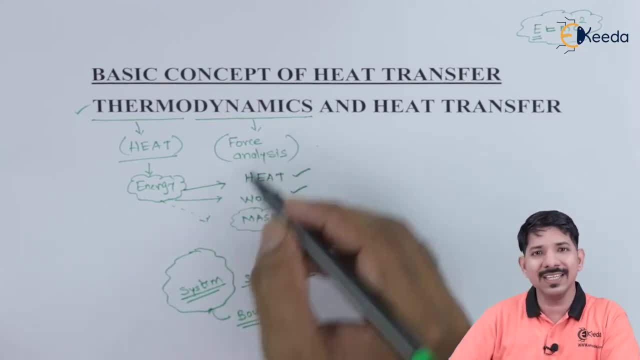 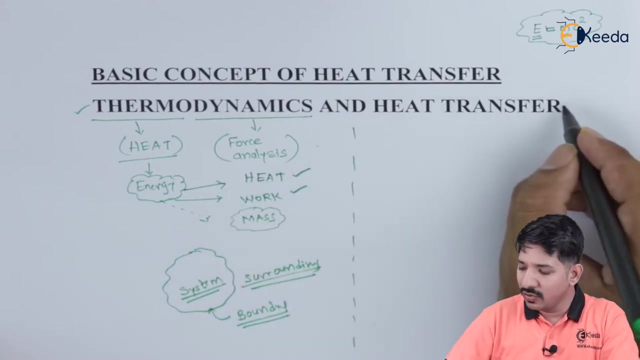 are happening across the boundary is what we have studied in thermodynamics. But in thermodynamics we did not talk about the mode of heat transfer and then the rate of heat transfer. These are the two important things that we are going to look into. the subject called 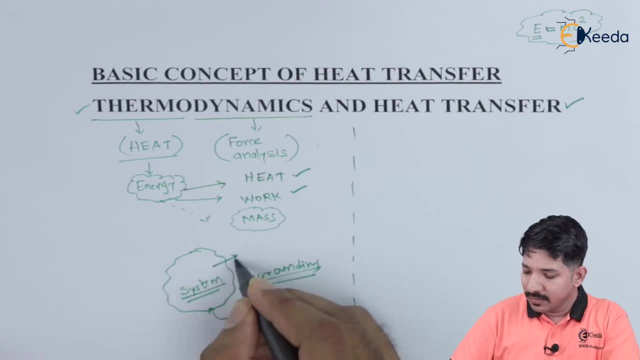 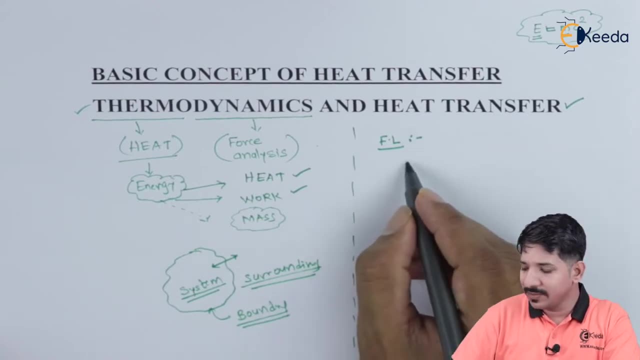 heat transfer. See, if you remember the first law itself, say, which is basically conservation of energy, E1 minus E2 plus E generated. or you can write: E in minus E, out is equal to delta E. that was my conservation of energy equation. This we try to convert into the first law of thermodynamics, which is basically the E. 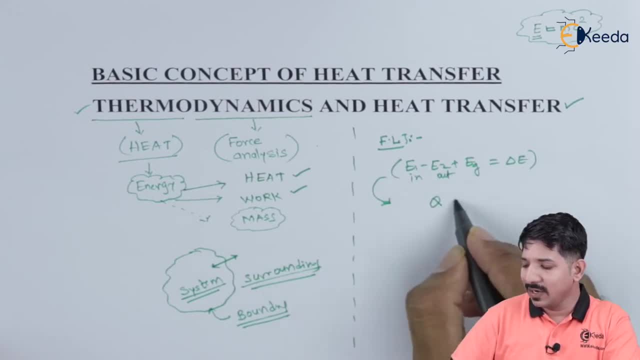 in, we try to imagine in the form of heat, and E out, we try to imagine in the form of work. There is no E generated that we have. This is what we call as the change in total energy. So this is my first law of thermodynamics. 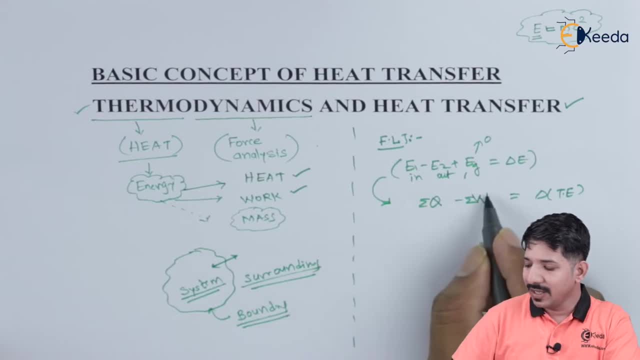 So, instead of one heat and one work, we try to write down the summation of heat and the summation of work. So basically, if there is a heat transfer from the system to the surrounding, or may be a work transfer from the system to the surrounding, what we get to know is nothing but the total. 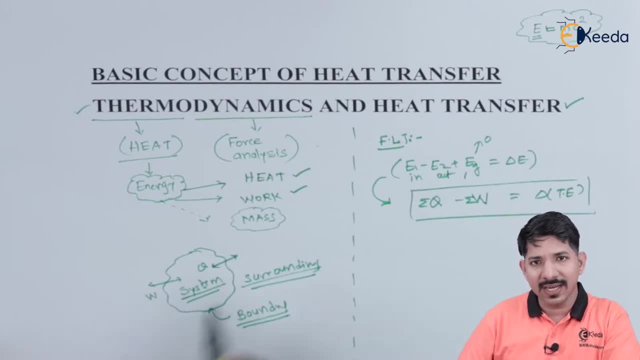 change in the energy- Energy of a system. that was the ultimate thing, But in this case we are not going to bother about the time. parameter means if the heat is transferring from system to the surrounding, we will not take care of what is the rate of heat transfer. 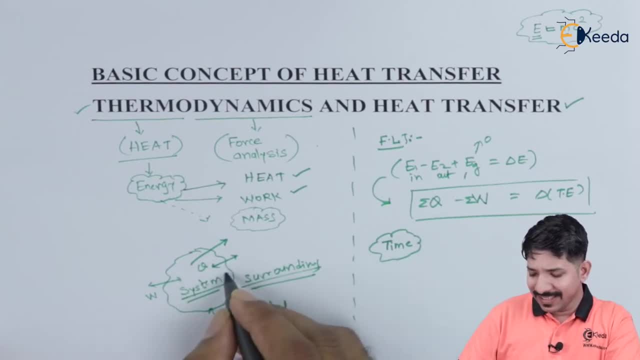 So what time it is required for transferring. let's say, let us give some number, let's say 100.. 1000 joule is what the energy that the system is giving to the surrounding. Now we are not going to bother about what time is required for the system to lose the 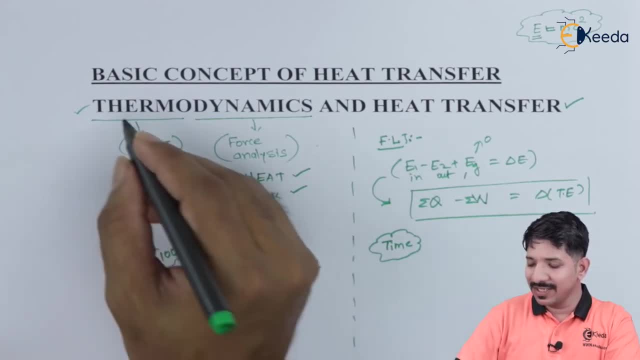 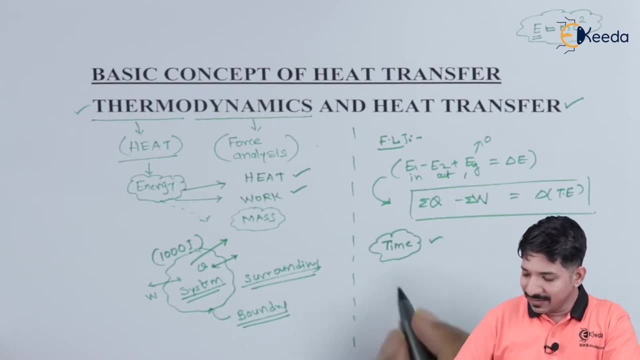 heat to the surrounding. This is what we have studied in thermodynamics. But in heat transfer we will be bothered about the time parameter. That is why, if you see, we used to write: when we talk about heat, Heat- In the thermodynamics, we used to write this as capital Q, which is basically an intensive 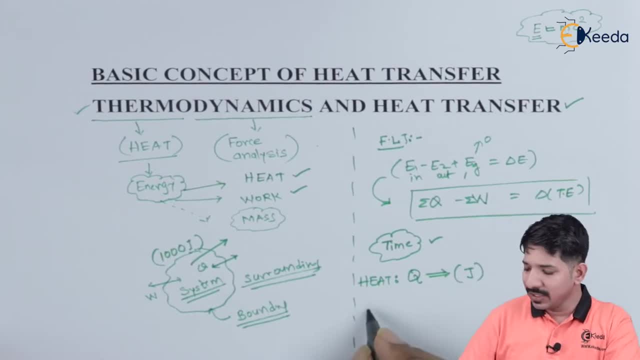 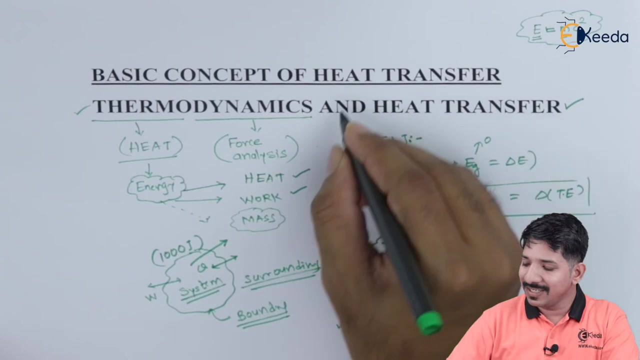 property and the unit was always a joule. that is the SI unit. But in case of heat transfer, we will not talk about heat itself, we are going to talk about heat transfer. Why we are going to talk about heat transfer? why the subject name itself is heat transfer. 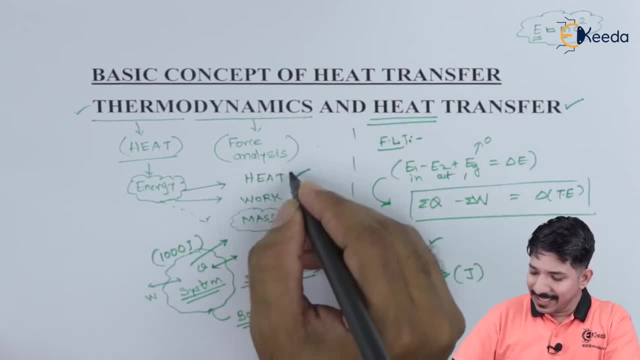 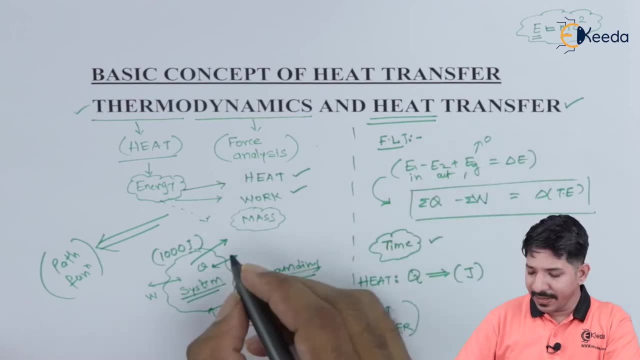 why not only heat? because this heat and work both of them are, Since both of them depend on the path that is followed. they always exist at the boundary. neither a system nor a surrounding can have a claim of having a heat or work. They can only have a claim that I am losing so much of amount of heat or so much of amount. 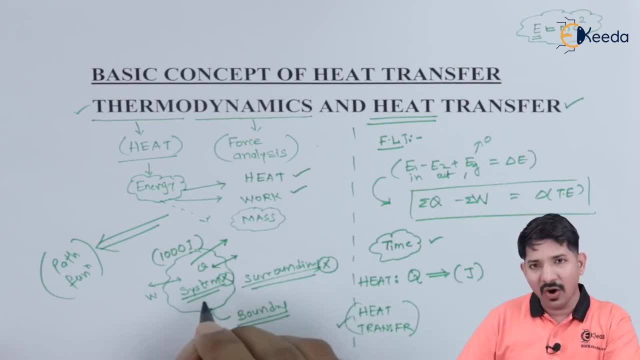 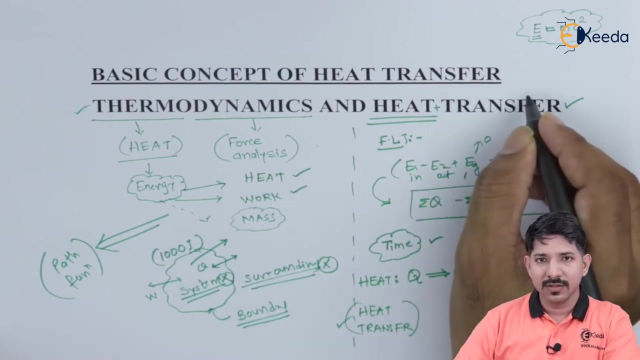 of work or I am gaining so much amount of heat or so much of amount of work. The heat and work can only be seen at the boundary, neither at the system nor at the surrounding. That is why the heat has to be clubbed with the transfer term. 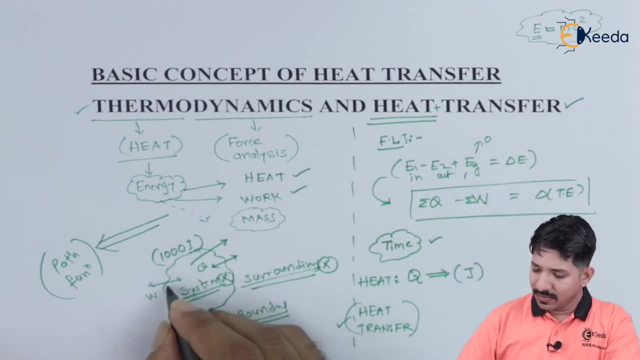 That is why the name itself is a heat transfer, because we can only find heat at the boundary. Now, in the thermodynamics we talked about heat, the unit was joule and in case of heat transfer, we are not going to talk about heat, but the rate of heat transfer. 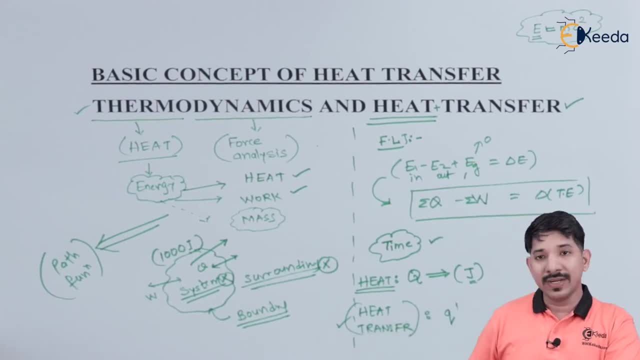 So that is why the indication is Q dash. Q dash talks about the rate of heat transfer, or you can write this as capital Q dash, and obviously the unit is joule per second, which is Watt. So this is the major difference. This is one of the major difference that we have in case of thermodynamics and heat transfer. 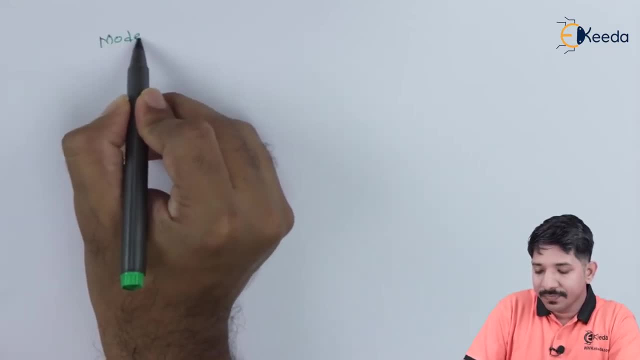 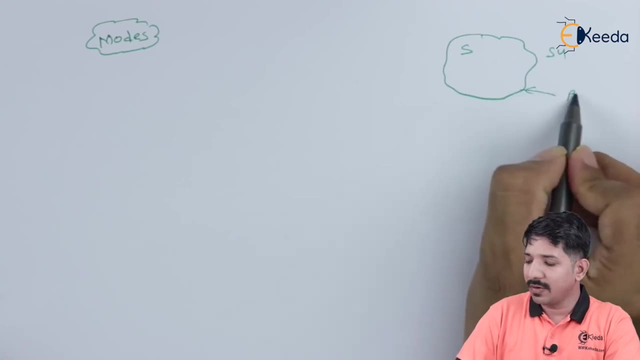 The other difference is mode. So again, if there is a system and this is the surrounding, Let's say this is a boundary. If I say that heat is transferred from the system to the surrounding, let's say my heat is again thousand joule. 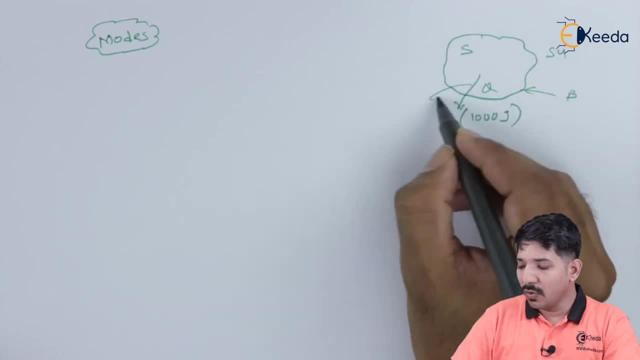 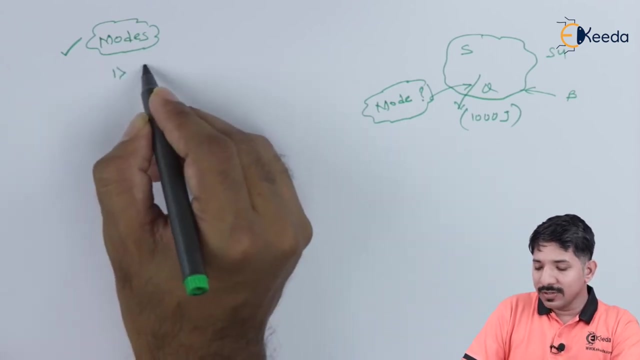 Now we will not concern about in what mode the heat is getting transferred from the system to surrounding. This was there in thermodynamics. but in case of heat transfer we have to consider the modes. So all of us know that there are basically three modes. 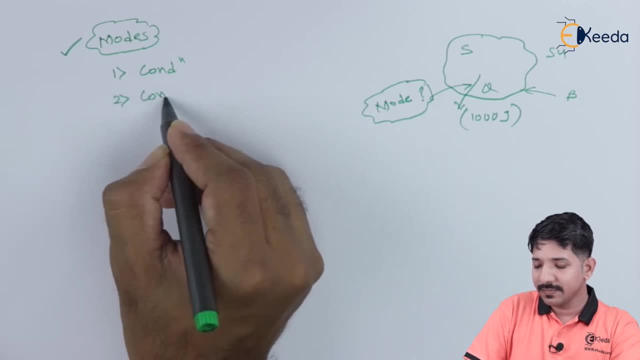 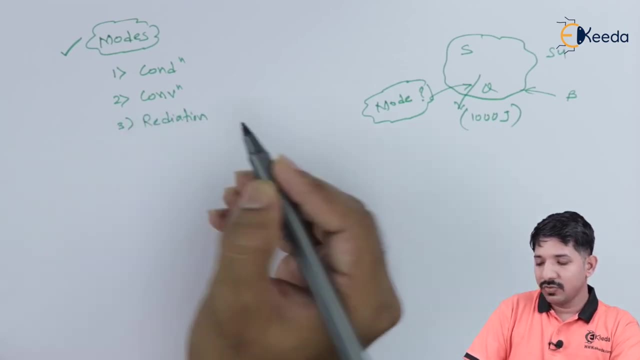 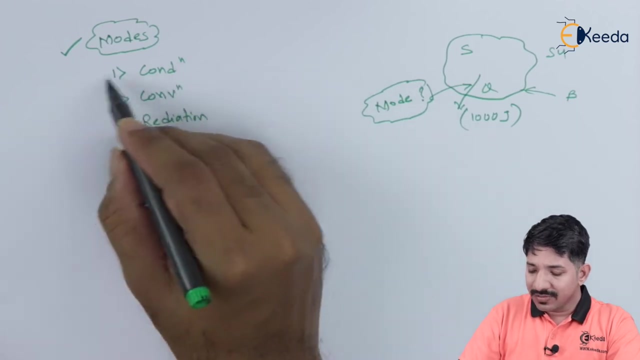 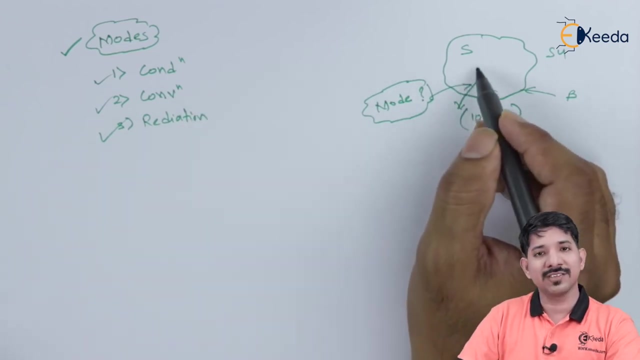 That is, conduction, convection and radiation. So these are the three modes by which the heat can transfer from the system to surrounding. We are going to see to it which mode is followed, or which combinations of modes are followed, while transferring heat from the system to surrounding. 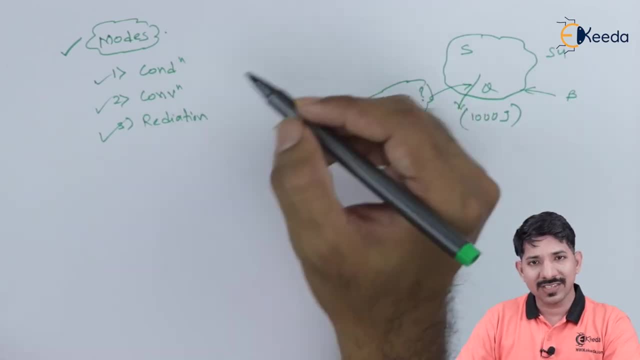 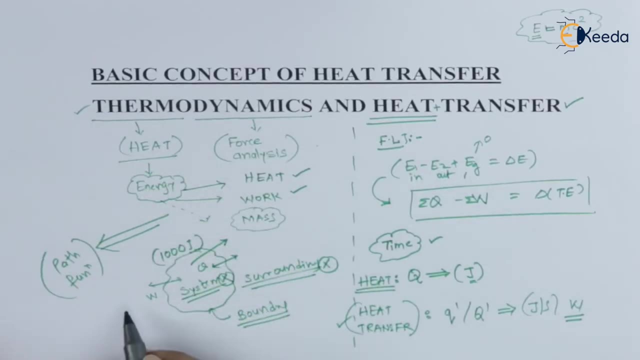 So these two are the major differences between what we have studied in thermodynamics and what we are going to study in heat transfer, Again in case of thermodynamics, the third part. So let me write down here: time was the first, then mode was the second and the third one.